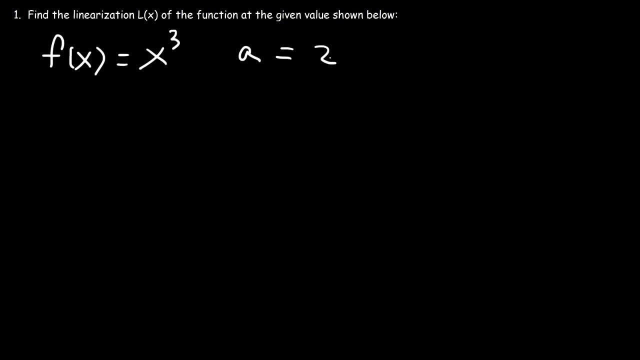 So, basically, what we really are trying to do is we're looking for the tangent line equation when x is 2.. That's the basic idea of what we're doing, And you could use this formula: L of x is equal to f of a plus f, prime of a times x minus a. 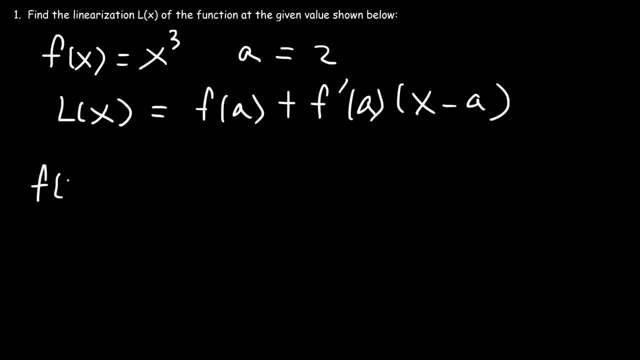 Now what is f of a? And we know a is 2,, so f of 2, we just got to plug it into this equation And that's going to be 2 to the third power. So 2 times 2 times 2, that's 8.. 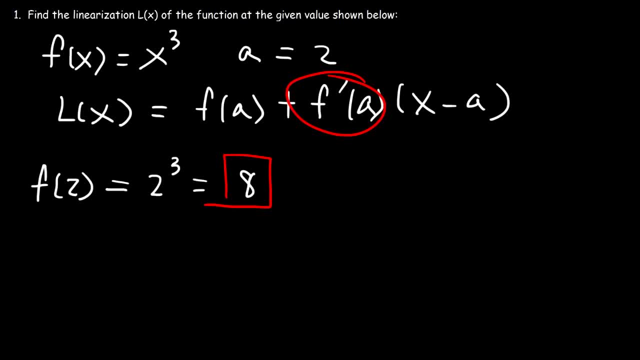 Now we need to calculate f prime of a Or f prime of 2.. To do that we need to find the first derivative. So the derivative of x cubed used in the power rule is 3x squared, And so f prime of 2 is going to be 3 times 2 squared. 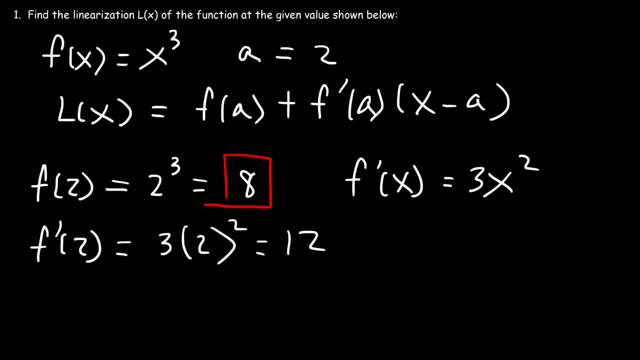 2 times 2 is 4, times 3,, that's 12.. So once you have f of a and f prime of a, you're now ready to plug in everything into this equation. So l of x is going to be f of a, which is 8, plus f, prime of a, which is 12, times x minus a, and a is 2.. 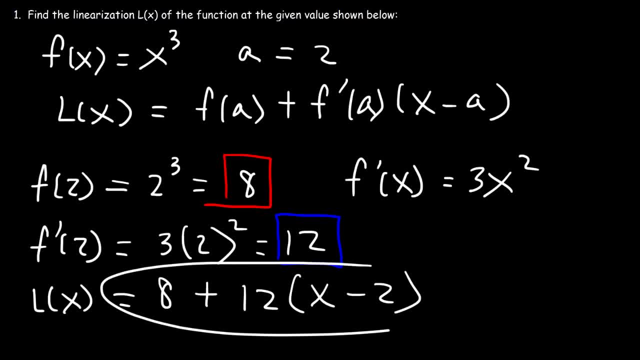 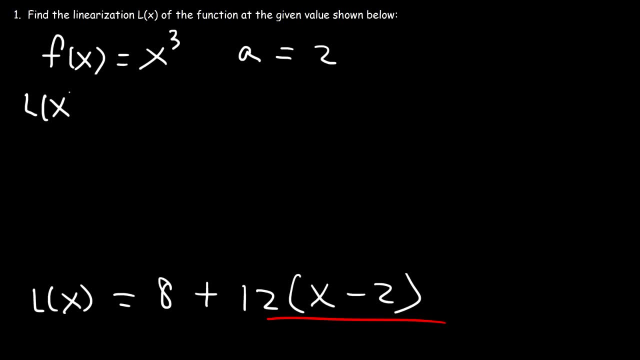 Now, at this point, all we need to do is simplify this equation. So let's distribute 12 to x minus 2.. But first I need to make some space, So let me get rid of a few things. So it's going to be 8, and then 12 times x, and then 12 times negative 2, which is negative 24.. 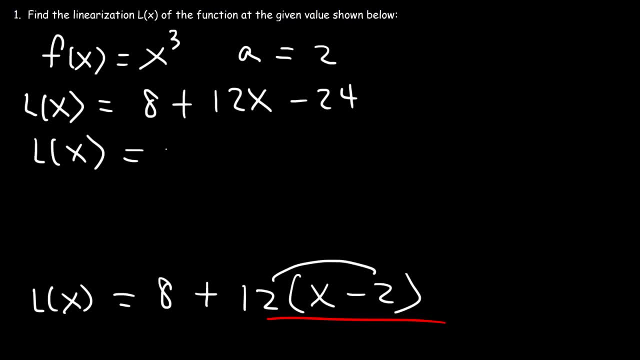 And so 8 minus 24, that's negative 16.. So l of x is going to be 12x minus 16.. So this is the linearization of the function when a is 2.. So that's the equation of the tangent line when x is 2.. 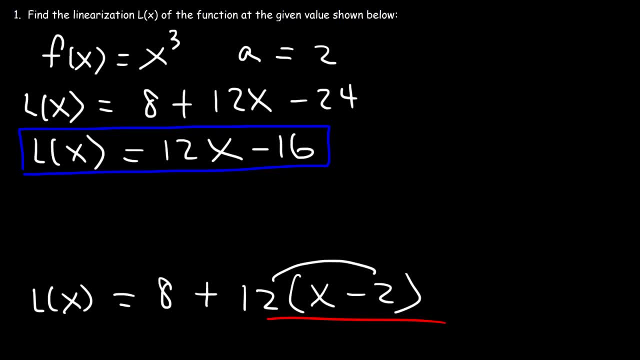 Now, one good thing of linearization is it helps us to approximate certain values. For instance, let's say, if we wanted to calculate or estimate the value of 1.99 raised to the 3rd power Without a calculator, this would not be fun. 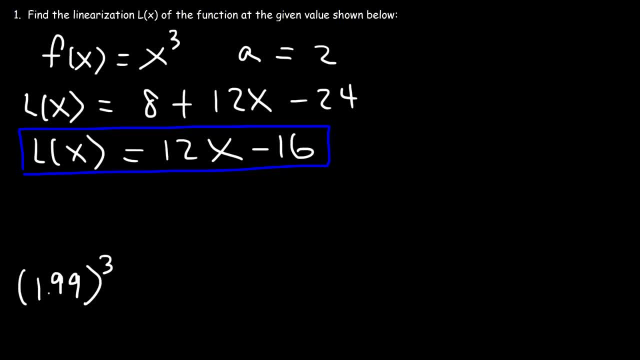 Now let's use a calculator. So 1.99 to the 3rd power. if you type that in, It's 7.880599.. That is the exact answer. But we can approximate this value using the linearization function at this particular number. 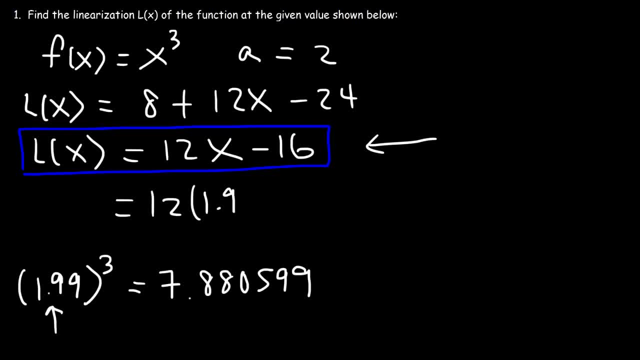 So it's going to be 12 times 1.99 minus 16.. Now let's see if we can do this without a calculator, Because if we have access to a calculator, We can simply type this in. So let me just get rid of this stuff. 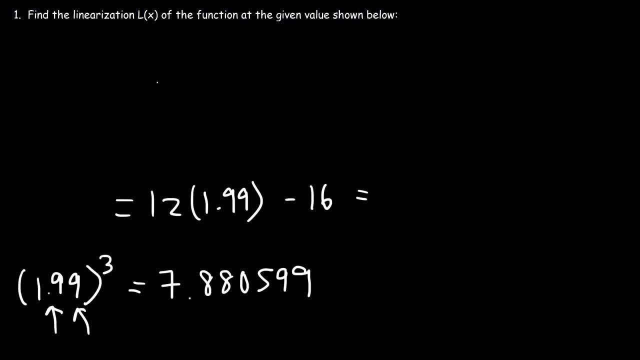 So what is 12 times 1.99? without a calculator, 1.99 is 2 minus 0.01.. And so 12 times 2 is 24.. And 12 times 0.01 is 0.12.. 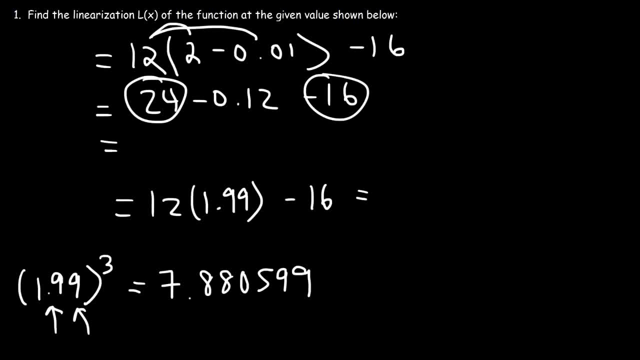 Now 24 minus 16 is 8. And 8 minus 0.12 is 7.88.. Because 100 minus 12 is 88. So notice how close these two values are. So if you need to approximate some number, that is difficult to do without a calculator. 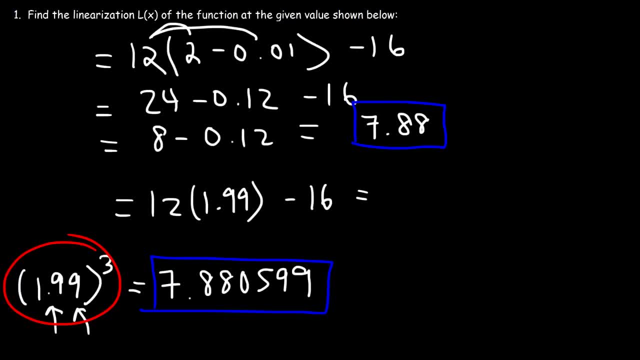 And if you know the function- in this case it's x cubed- You can approximate it with a linearization technique Without the use of a calculator, And so that's how this information can be applied in a typical setting. Now let's try another problem. 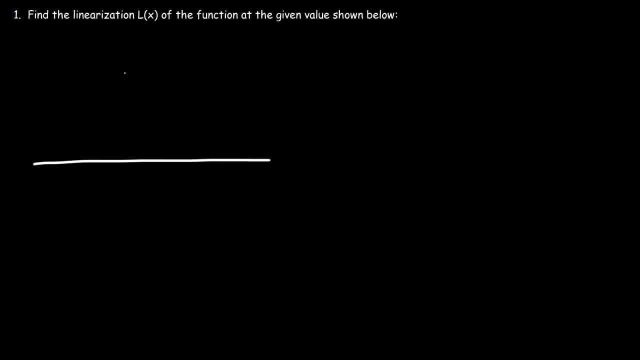 By the way, if you want to see a graph, This is the right side of the graph of x cubed, And the tangent line is basically a line that touches the curve at one point. And so you can, And so you can. 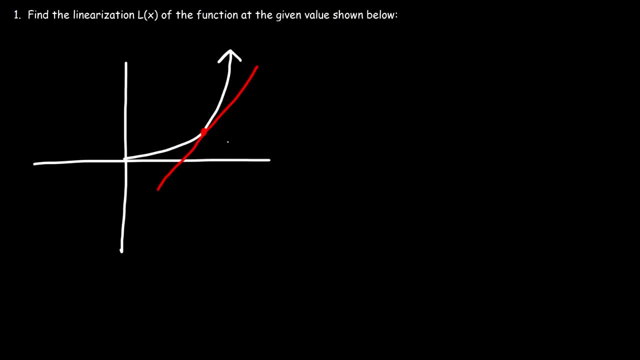 You can estimate a certain function value by using the tangent line, And the estimation works if the number is close to the point of intersection. In this case, a was 2. And so we wanted to estimate 1.99 raised to the third power. 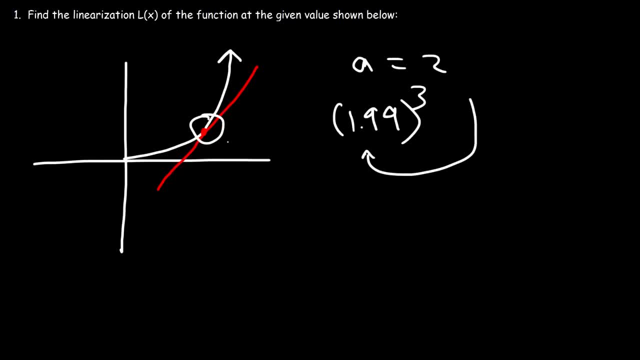 The reason why it works so well is because 1.99 is very close to 2. And so this point here, the point of intersection that's at x equals 2.. So you can use L of x to approximate function values when x is very, very close to 2.. 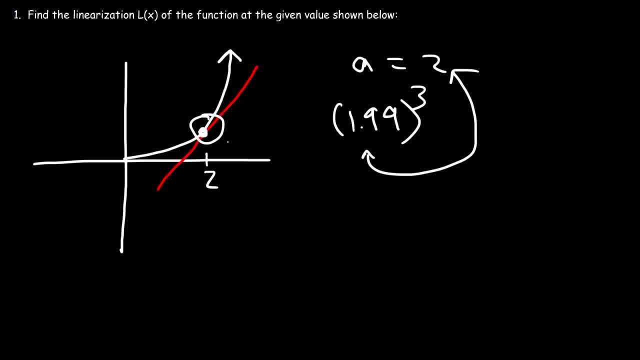 Because that's where the tangent line meets the curve. If you try to approximate, let's say, 2.99.. You can't use 2 as a value, You have to use 3.. So you need to create a new tangent line when x is 3.. 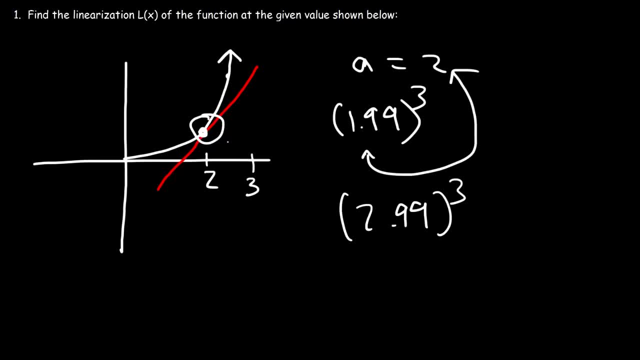 And so, basically, whenever you want to estimate a number Using this process, These two numbers have to be very close, Otherwise the accuracy will be lost. You won't get a good estimation. Now let's try this problem. Let's say that f of x is equal to the square root of x. 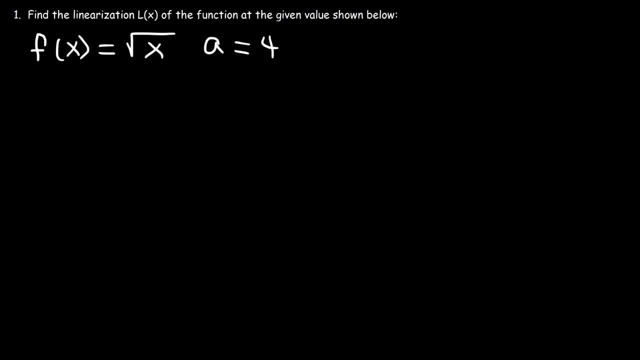 And a is 4.. So find the linearization L of x of the function at the given a value. In addition, Once you have that, use it to estimate the square root of 3.99.. So first let's determine f of a. 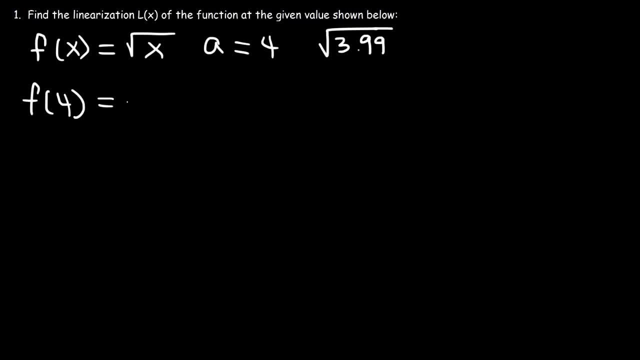 Or f of 4.. So f of 4, that's the square root of 4. That's equal to 2.. Next we need to determine f prime of a. So first we need to calculate f prime of x. 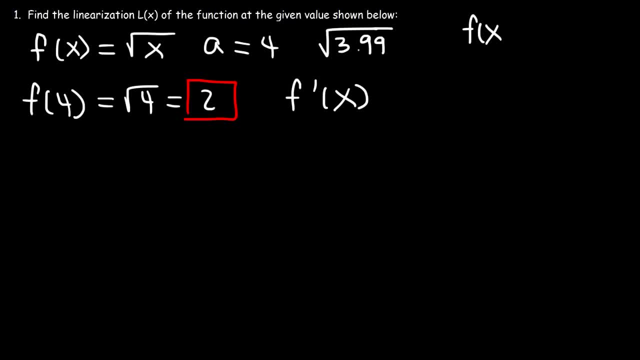 Now f of x, which is the square root of x. If we rewrite that, that's x to the 1 half. So using the power rule, it's going to be 1 half: x to the 1 half minus 1, which is negative 1 half. 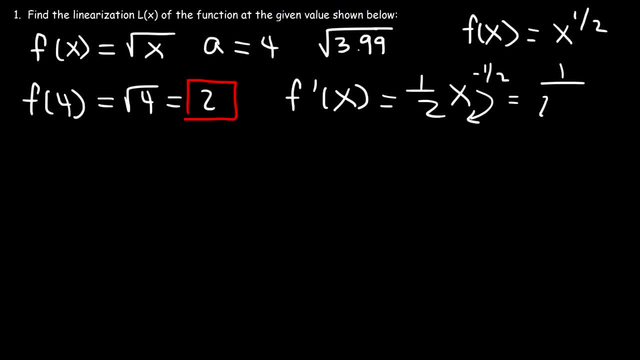 And then if we bring the x to the bottom, it's going to be 1 over 2, x to the 1 half, Which is the same as 1 over 2 square root x. So now f prime of 2, I mean f prime of 4 rather, because a is 4.. 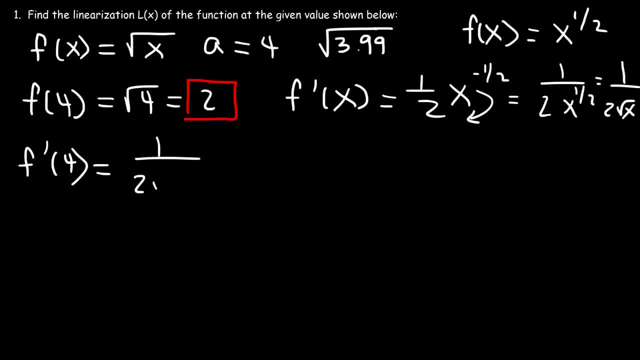 That's going to be 1 over 2 times the square root of 4.. And the square root of 4 is 2. And 2 times 2 is 4.. So f prime of a is 1 over 4 in this example. 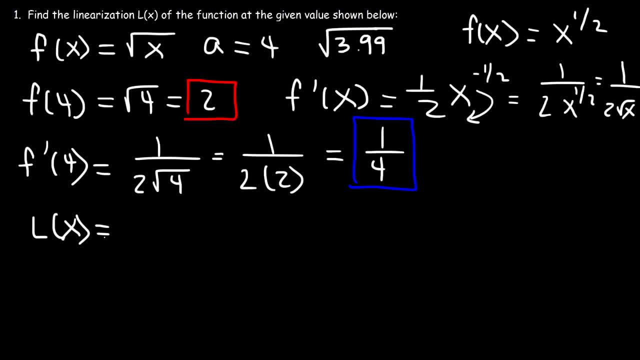 So now let's rewrite the linearization function l of x, And we said that was f of a plus f prime of a times x minus a. So f of a in red is 2.. f prime of a is highlighted in blue. 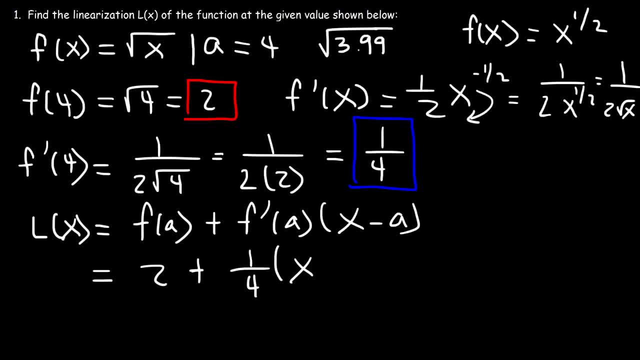 That's 1 over 4.. And a is this number which is 4.. So that is the linearization function, And you could simplify it if you want to, But when estimating this number, I'm going to use this form. 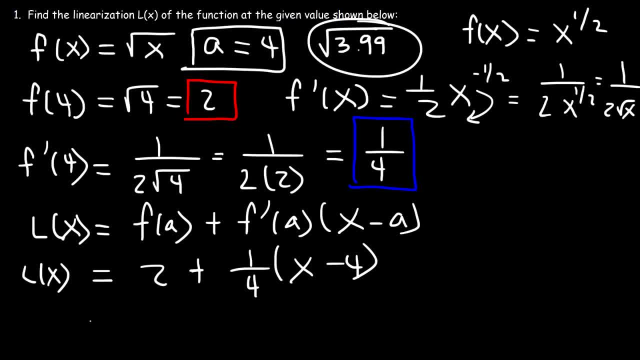 Now, if you want to simplify it, this is what you're going to get. It's going to be 2 plus 1 fourth x, and then 1 fourth times negative 4.. That's going to be negative 1.. And so 2 minus 1 is 1.. 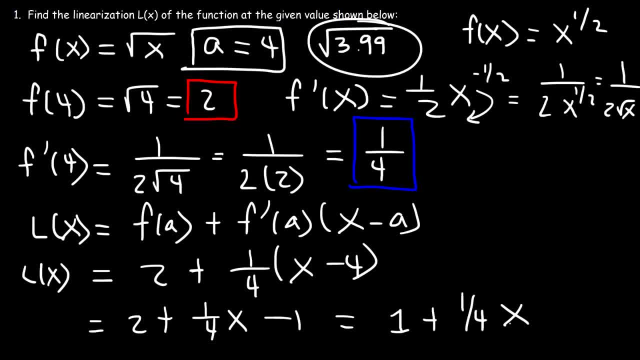 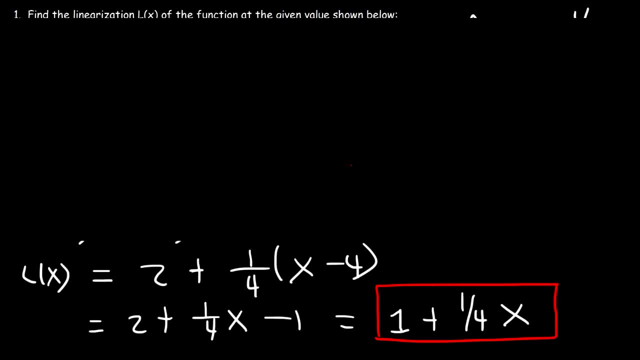 So it's going to be 1 plus 1, fourth x. So that's the simplified version of l of x. That's what it equals, Thank you. Now let's estimate the square root of 3.99.. So first let's get the exact answer with a calculator. 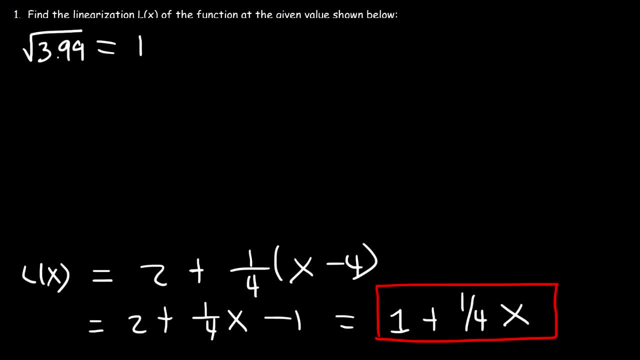 So if you type it in, this is equal to 1.997498436.. Those are the numbers that my calculator gave me. So now let's use l of x. Now you have to decide if it's easier to use this form or this form. 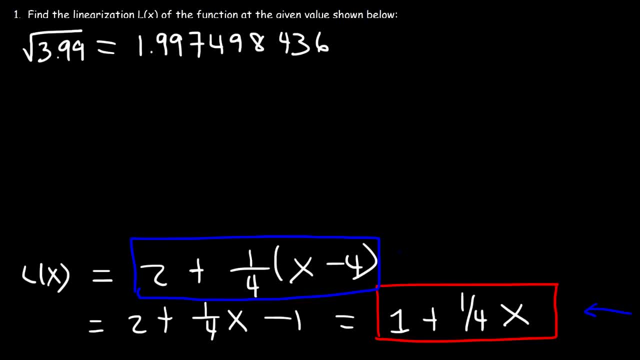 What do you think? I think it might be easier to use this form, But in the end- I mean both- will still be the same. So let's calculate l of 3.99.. So it's going to be 2 plus 1, fourth times 3.99 minus 4.. 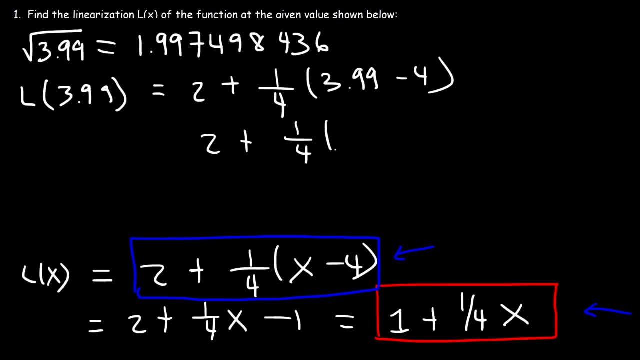 Now 3.99 minus 4, that's negative 0.01.. Now 1 over 4 as a fraction, or rather as a decimal, is 0.25.. Now, if you're not sure about that, you can use long division. 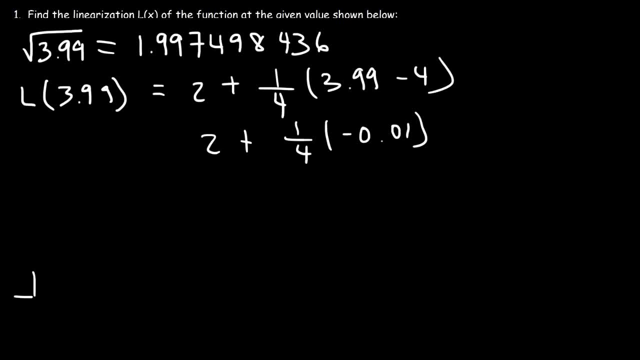 Anytime you need to convert a fraction to a decimal, So the numerator goes on the inside. Now, 4 goes into 1 zero times, So we need to add a zero on the decimal point. 4 goes into 10 two times. 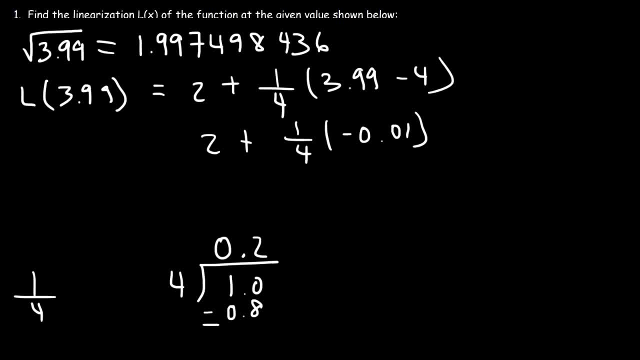 4 times 2 is 8. And 4 times 0.2 is 0.8.. 10 minus 8 is 2.. Add a zero, 4 goes into 25 times. with no remainder, I'm running out of space. 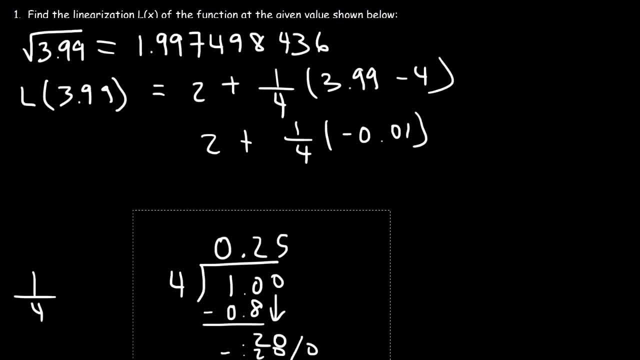 So you get 0.25.. 0.25.. So we have 0.25 times negative. 0.25 times negative is 0.01.. Now, what is 0.25 times 0.01?? Well, let me help you to understand it. 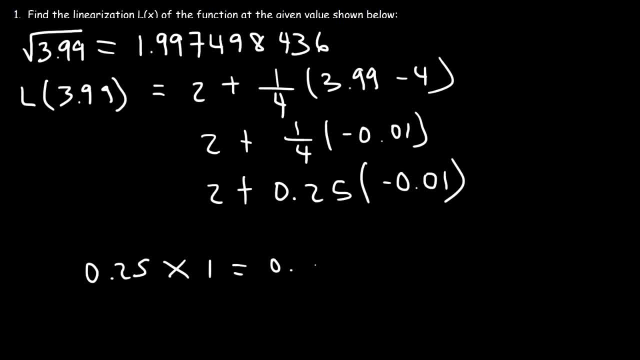 So 0.25 times 1 is equal to itself. If we multiply it by 0.1, it's going to be 0.025.. You just got to move the decimal point, And then, if you multiply it by 0.01, you got to move the decimal point by two spaces. 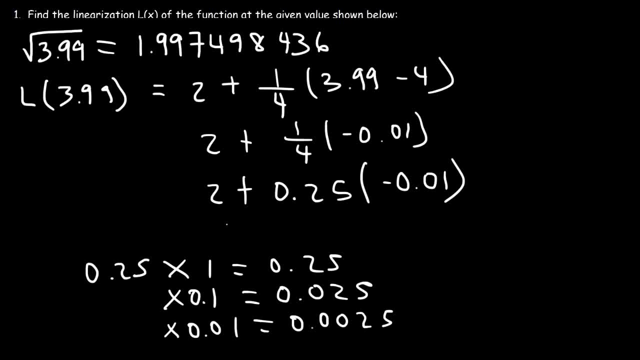 So it's going to be 0.025.. 0.025.. 0.025.. 0.025.. 0.0025,, which is what we're going to have. So this is 2 minus 0.0025.. 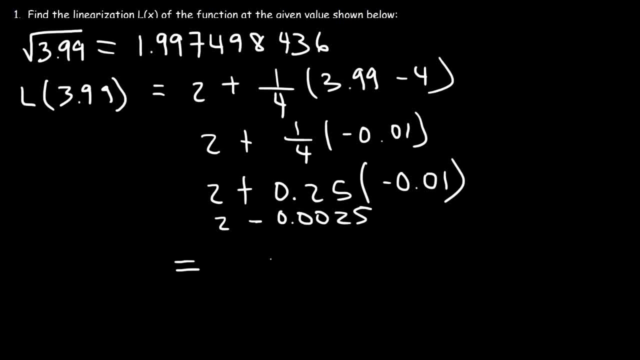 2 minus 0.0025.. That's going to be 1.9975.. For those of you who are not sure, you can subtract these numbers the old-fashioned way, So this is 2, and we're going to subtract it by 0.0025.. 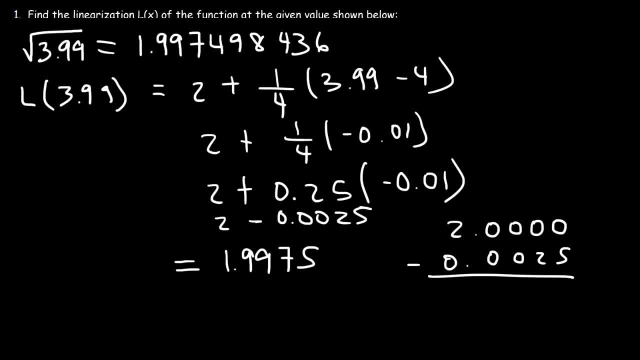 0.0025.. 0.0025.. So first we need to borrow a 1, so that this becomes 10.. Now we need to take away a 1 from this one, So this becomes a 9,, a 9, and a 9.. 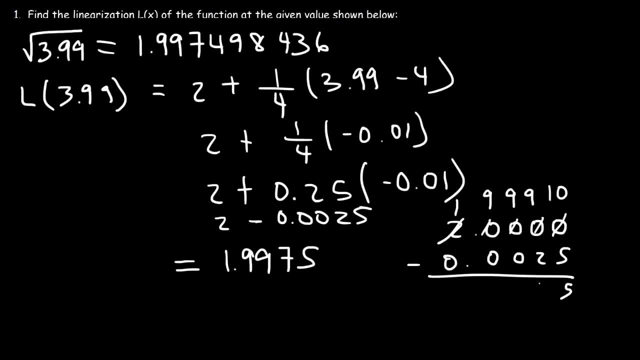 So 10 minus 5 is 5.. 9 minus 2 is 7.. 9 minus 0 is 9.. 9 minus 0, that's 9. again, 1 minus 0 is 1.. Now, if we compare these two numbers,